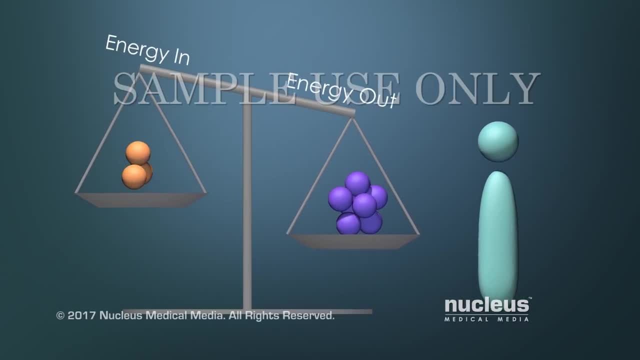 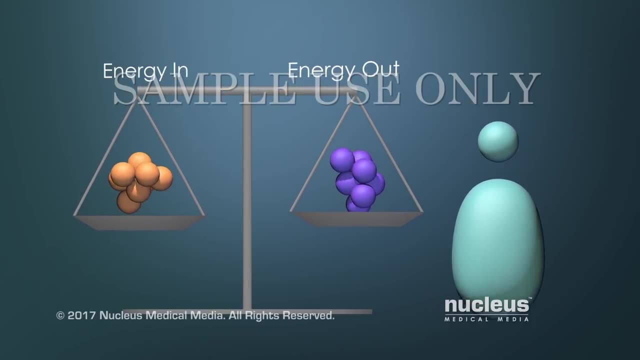 energy in is less than your energy out, you will lose weight. If your energy in is about the same as your energy out, your weight will stay the same. If your energy in is greater than your energy out, you will gain weight. Risks for becoming obese include an inactive lifestyle. lack of access to places to exercise. lack of access to healthy food, a diet rich in high-calorie, fatty and sugary foods, meals with oversized food portions, having a family history of being overweight or obese, diseases such as hypothyroidism and polycystic. 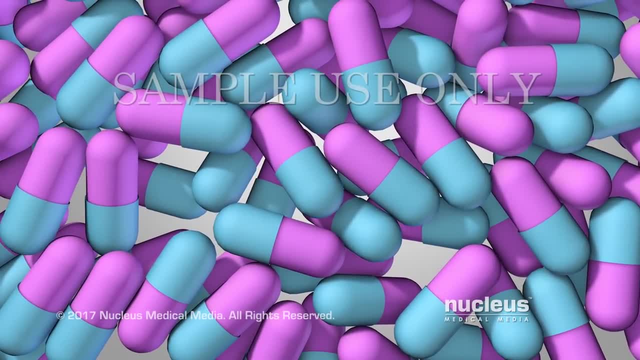 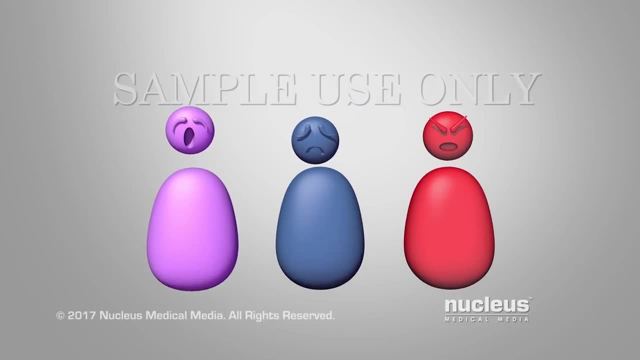 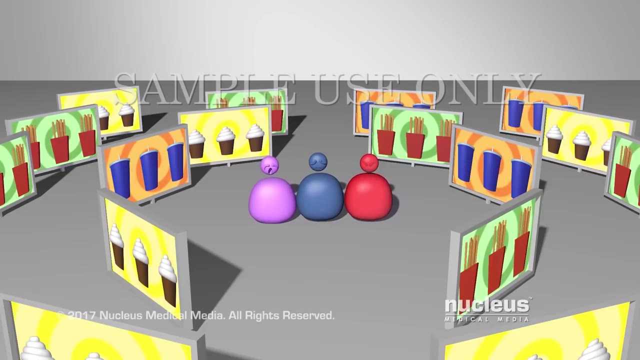 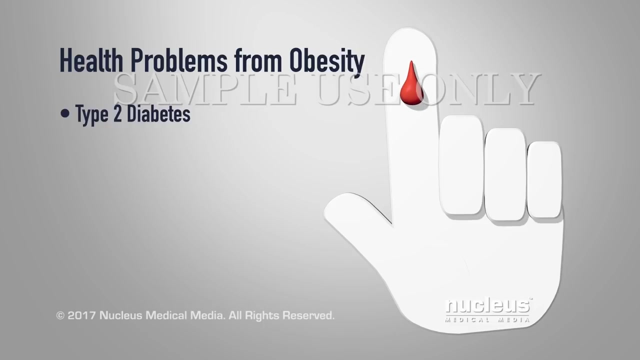 ovary syndrome, side effects from some medications, Lack of sleep, emotions that can make you want to eat more, and advertisements for high-calorie, unhealthy food and drinks. Obesity raises your risk of developing health problems such as type 2 diabetes, high blood pressure, high cholesterol, heart disease and diabetes. 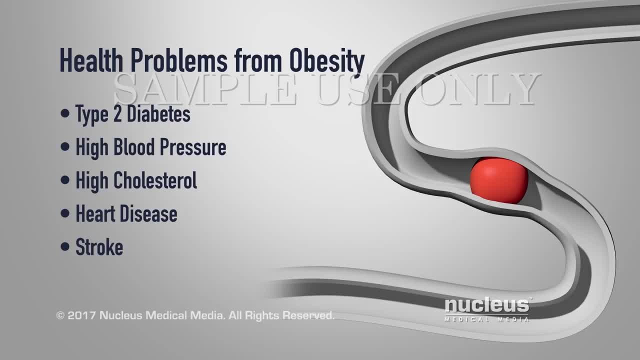 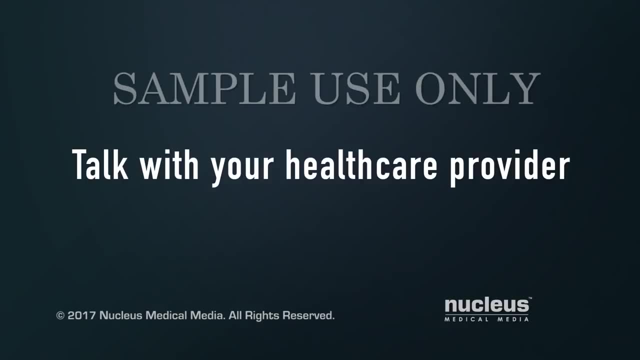 Obesity raises your risk of developing cancer, stroke and certain cancers. If you have questions about obesity, talk to your healthcare provider. 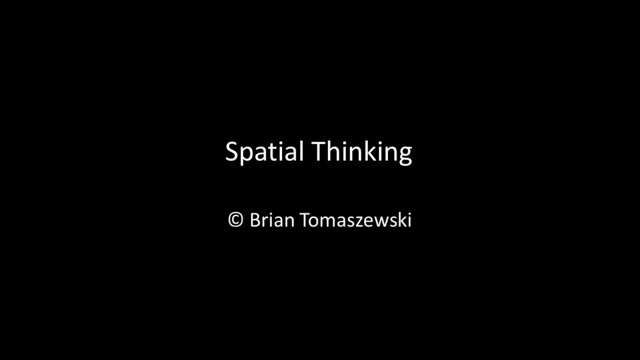 Hello and welcome to this lecture on spatial thinking. The learning objectives for this lesson are to understand what spatial thinking is and why it is important, and be familiar with spatial thinking support tools. Spatial thinking is a concept that is best illustrated with many examples, and in this lecture I will give you many examples of. 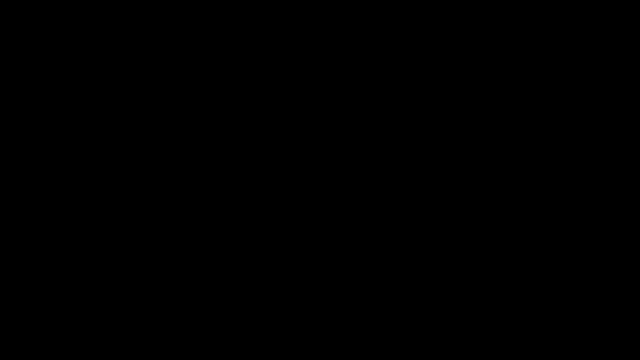 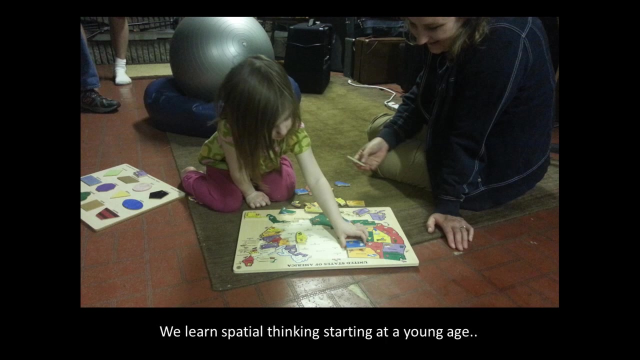 what is meant by spatial thinking. Spatial thinking is a skill that we learn starting at a very young age. In this picture, the young girl can be seen fitting shapes that represent US states into a puzzle. Behind her you can also see another puzzle that requires thinking. 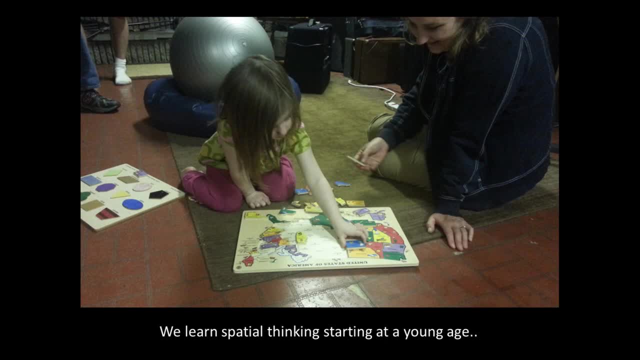 spatially about how shapes relate to one another. We use spatial thinking every day, whether we are aware of it or not. For example, counting using one's fingers, planning road trips and reasoning about travel distances using a map or using space as a